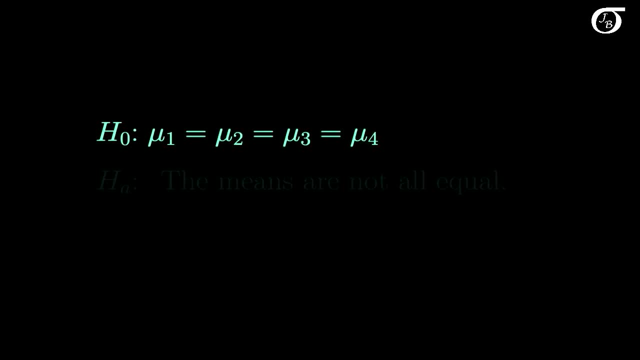 And here we're going to test the null hypothesis that the population means of the four groups are all equal against the alternative hypothesis that the null hypothesis is false, Or in other words, the alternative hypothesis is that the population means are not all equal. 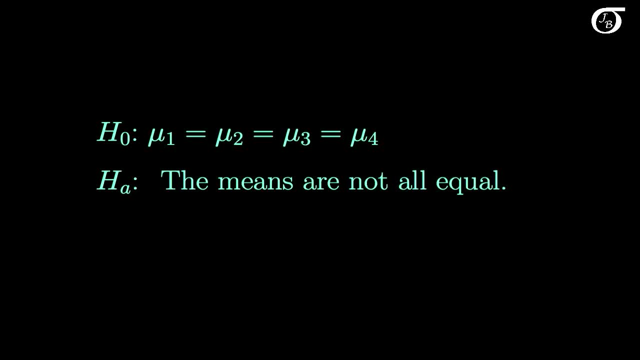 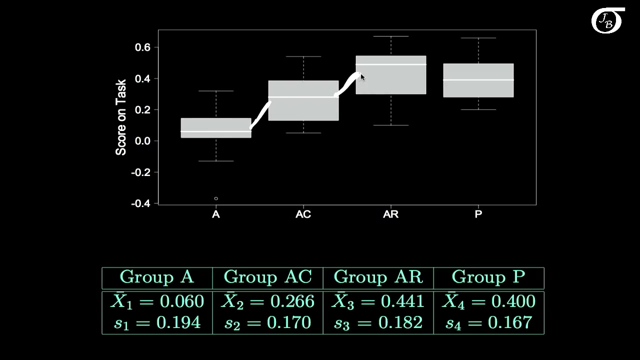 Now, because this is an experiment. the null hypothesis is sometimes written in terms of treatment effects. In other words, the null hypothesis might be written that the treatments have no effect. Here we have the box plots and the summary statistics. Visually, it appears as though there's differences between these groups. 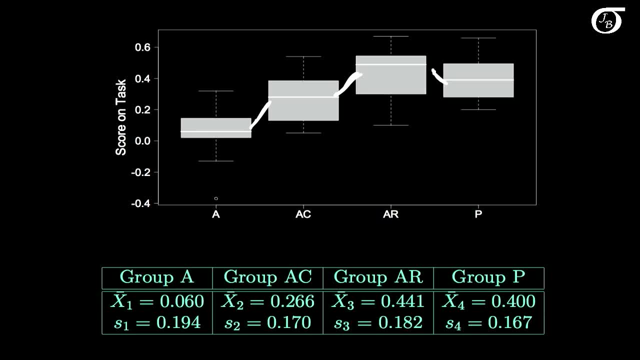 But what we want to do is test that statistically. Is there statistically significant evidence of a difference? The sample means for the four groups are listed down here, Also the sample standard deviations. The standard deviations are important for us because one-way analysis of variance assumes that 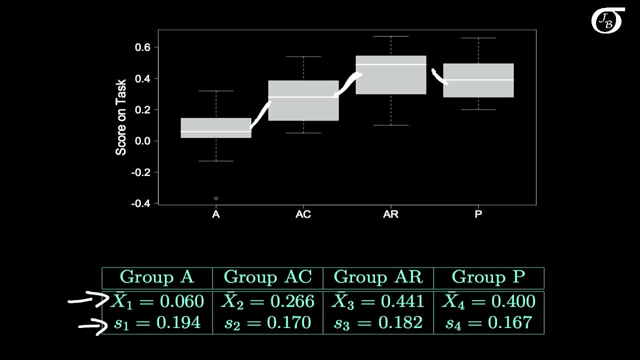 the population variances of the different groups are equal. If we look at the numbers down here, we see that the sample standard deviations are different, as they're going to be, but they're pretty darn close And visually it certainly looks like the variability within each group. 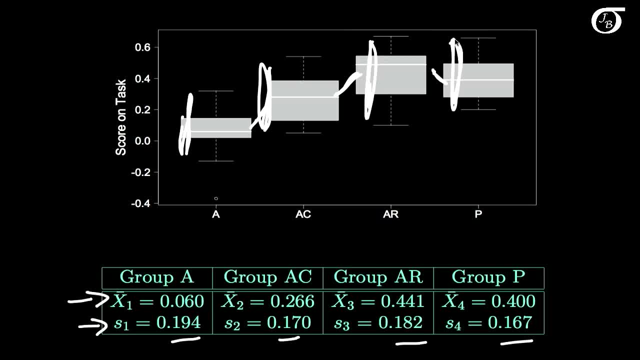 is pretty darn similar. not much going on there. So there's nothing to say that that assumption of equal population variances is violated here. There is one value here that's a bit of an outlier, but it's not too extreme and it's unlikely to have a massive influence on the results. 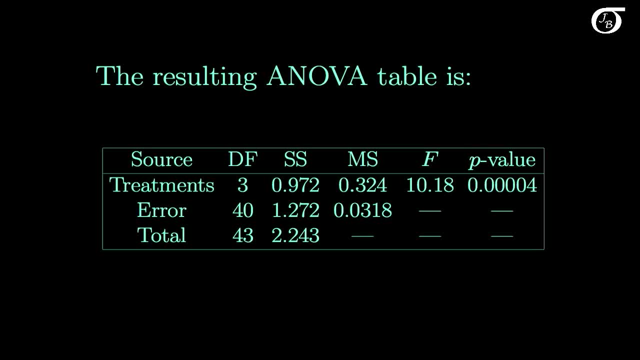 If we put our data into a computer and got our ANOVA table, it would look something like this: The calculations are possible to do by hand, but it's quite a bit of a hassle, so it's best to use a computer. 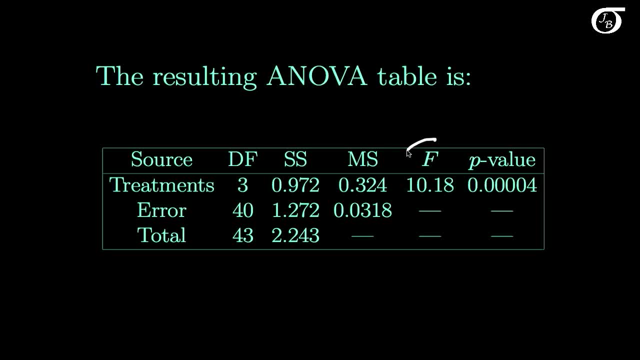 In the bitter end we get an F-test statistic. This is the F statistic that's testing the null hypothesis that the population means are equal. The p-value given here is the area to the right of this observed test statistic under an F distribution with 3 degrees of freedom in the numerator. 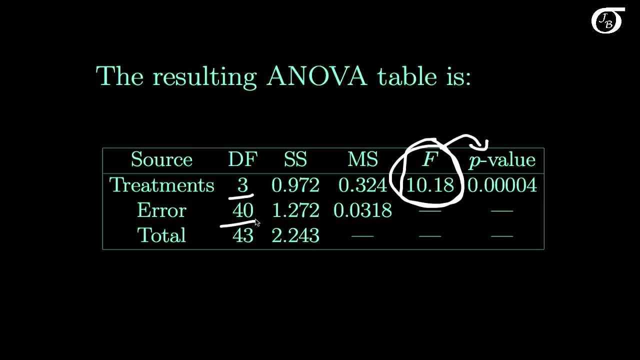 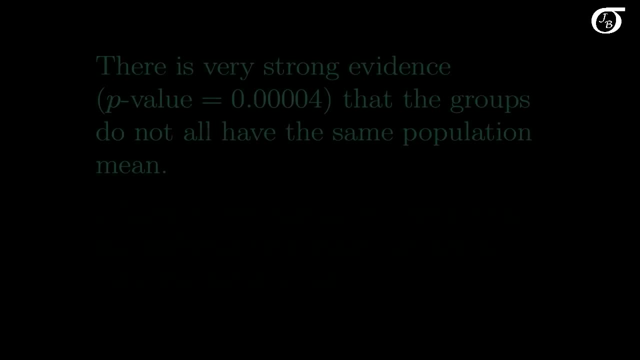 and 40 degrees of freedom in the denominator. This p-value is a very, very small value, and so there is very strong evidence against the null hypothesis. What does that mean in the context of this experiment? That small of a p-value says that there is very strong evidence.